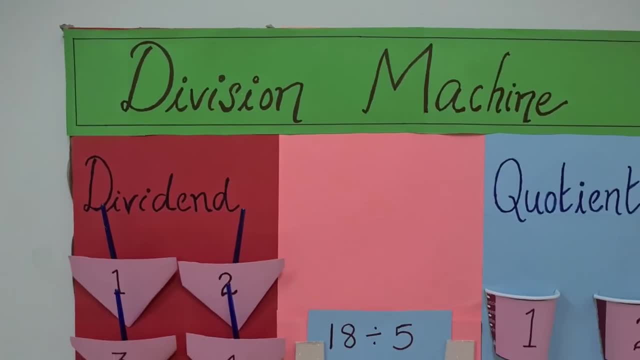 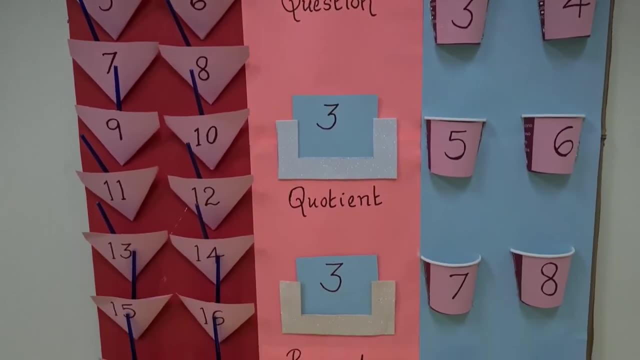 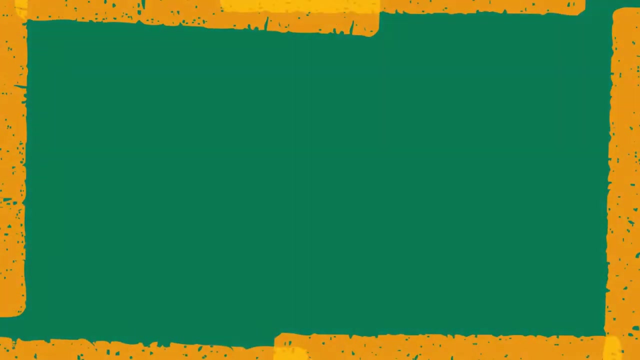 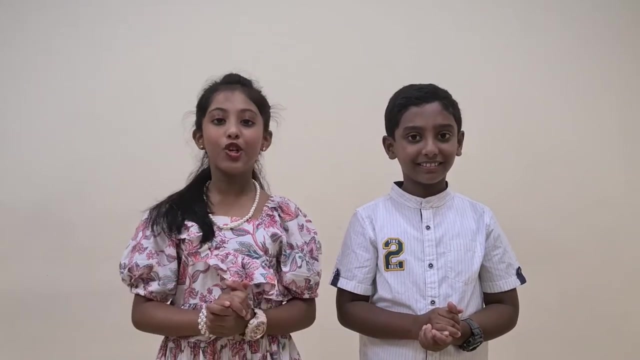 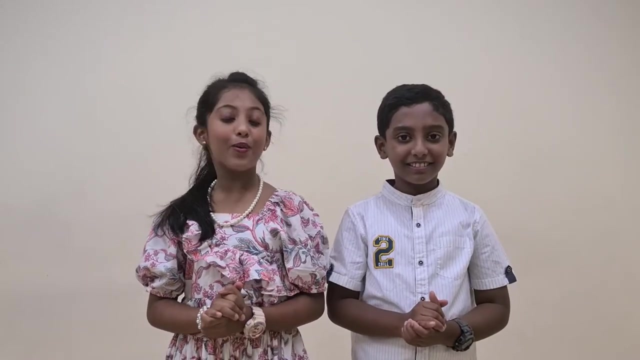 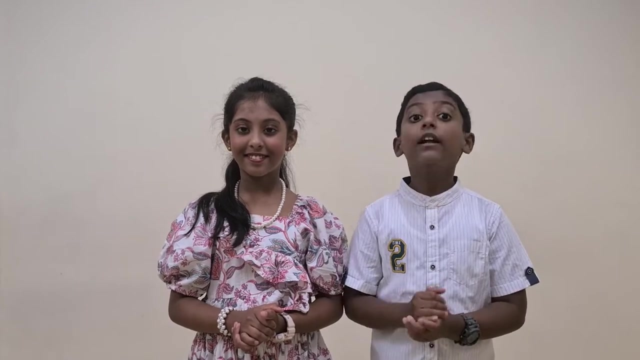 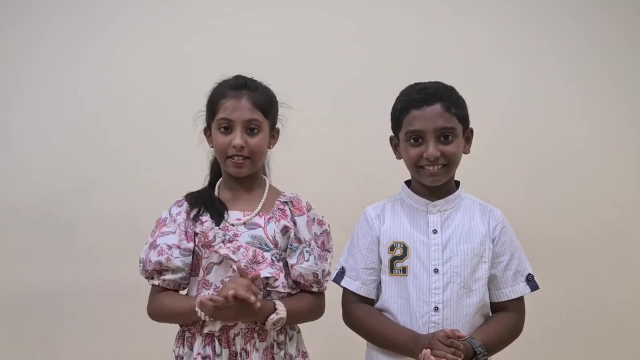 Hello guys, Once again, welcome back to our new video Hope you all have seen. I'm Joanna, I'm Joshua. Thank you everyone for supporting us Today we will do a math project on the topic division. Division is one of the four basic operations in mathematics. It involves the sharing of an amount into equal groups. 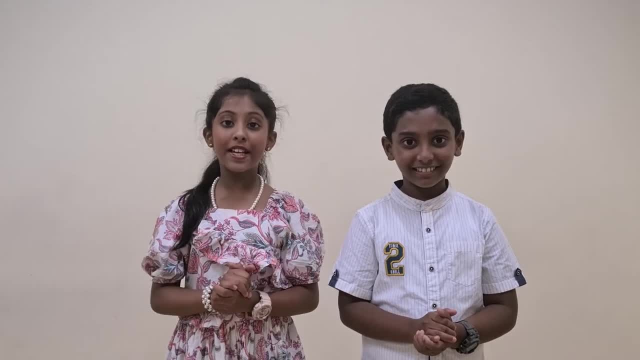 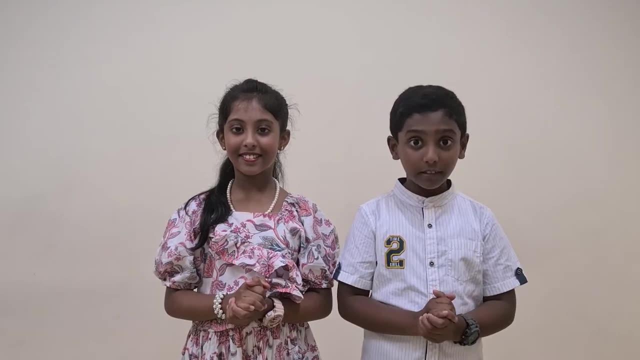 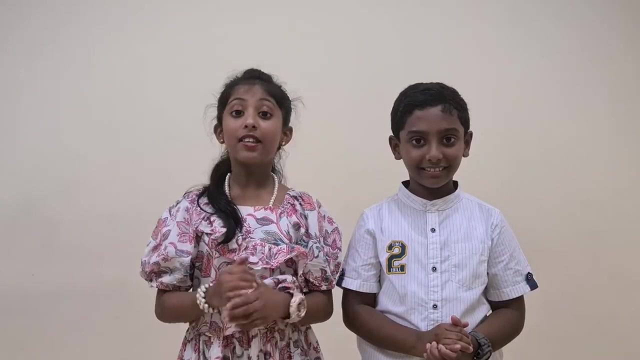 For example, 12 divided by 4 means 12 is shared into 4 equal groups. This problem: 12 is the divisor, 4 is the divisor and 3 is the quotient. In some cases, like 30 divided by 4, we cannot split 30 into equal groups. 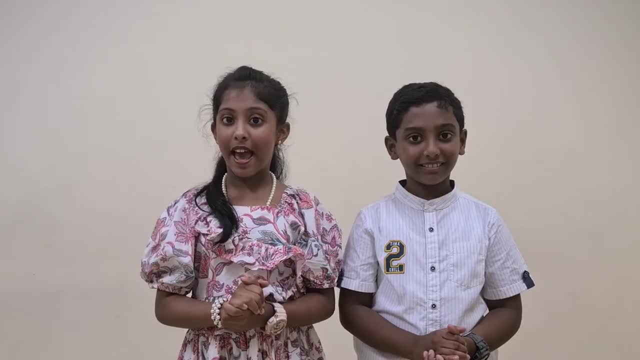 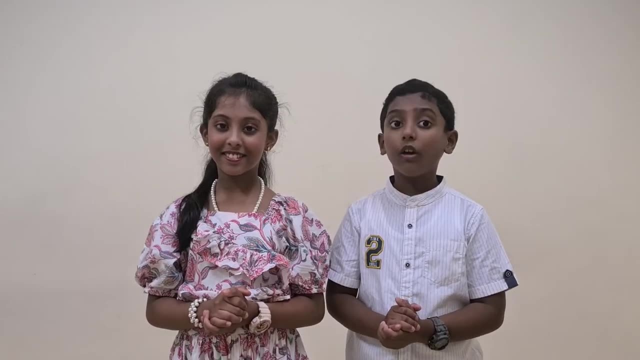 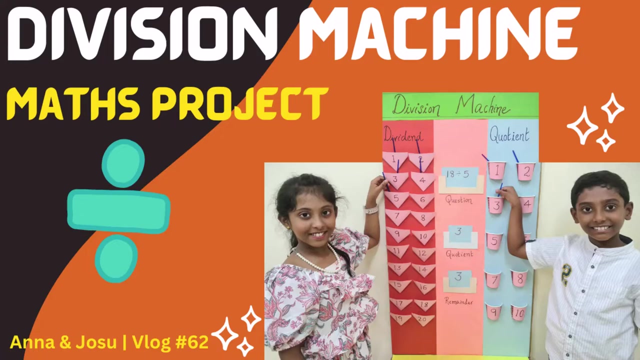 So we get 3 as the quotient and we get 1 as the remainder. Today we will do an easy way to practice division. Let's get started. Ok, Let's get into the video. Hello, Hello everyone, Woo. 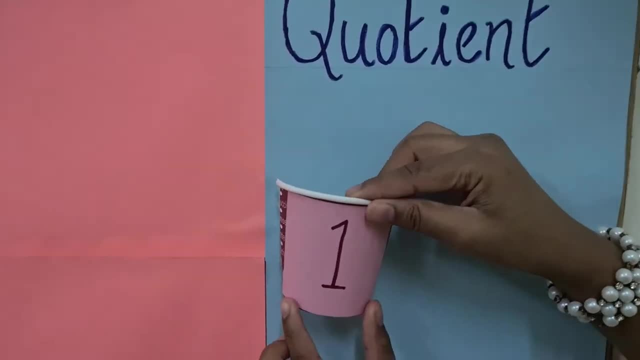 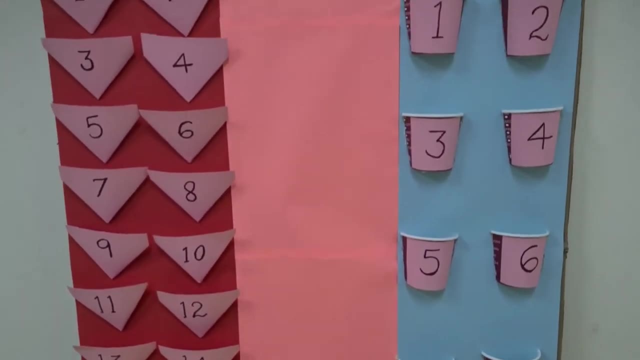 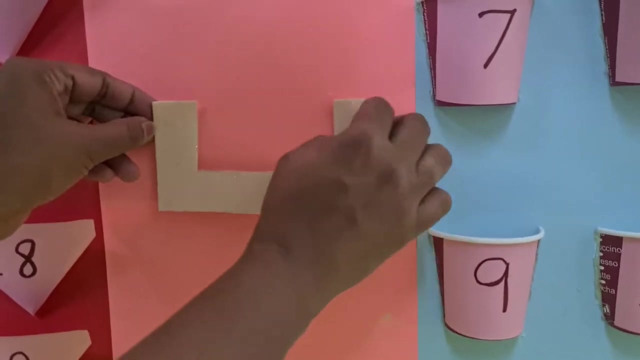 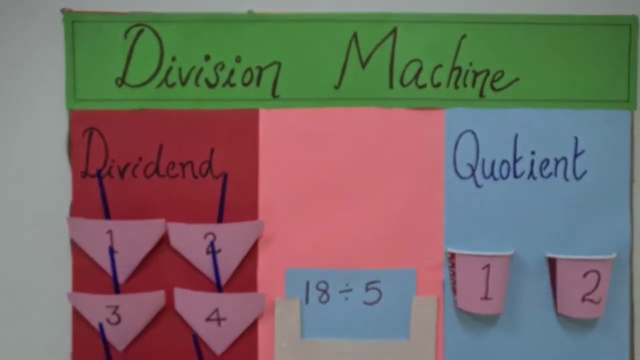 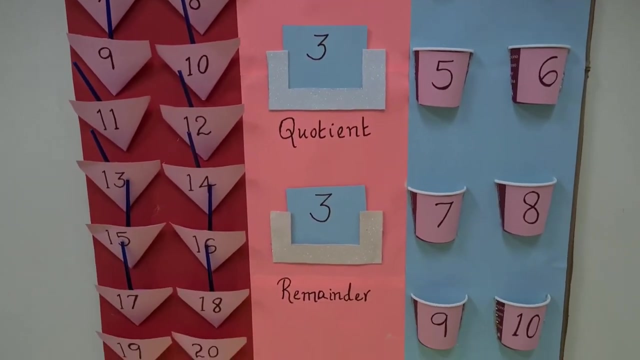 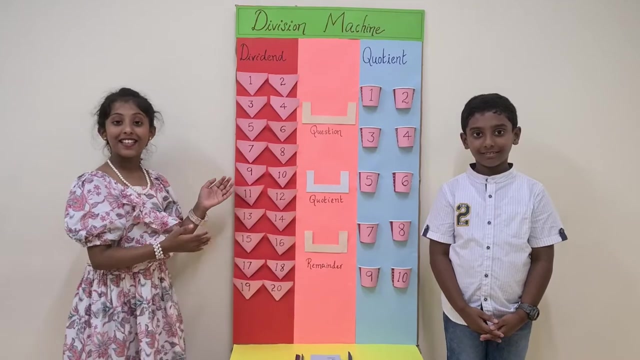 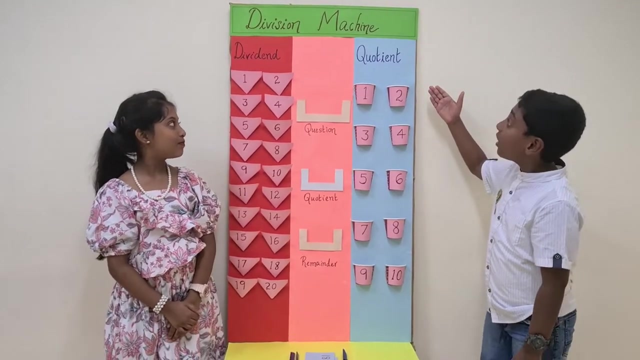 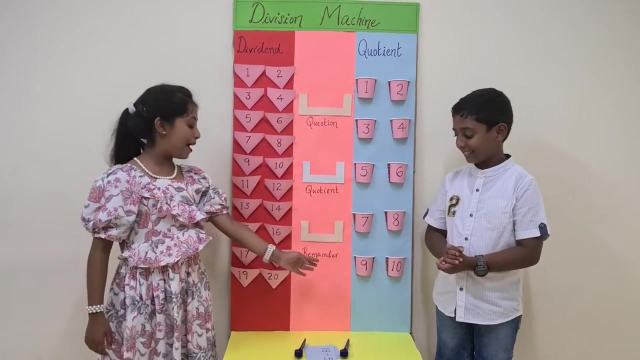 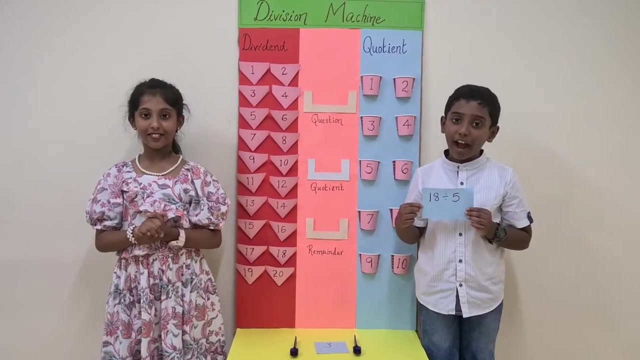 Woo, This is the division machine. These are the dividend pouches, These are the caution pouches. We have a question box, a caution box and a remainder box. Let's take a question 18 divided by 5. Let's put it in the question box.